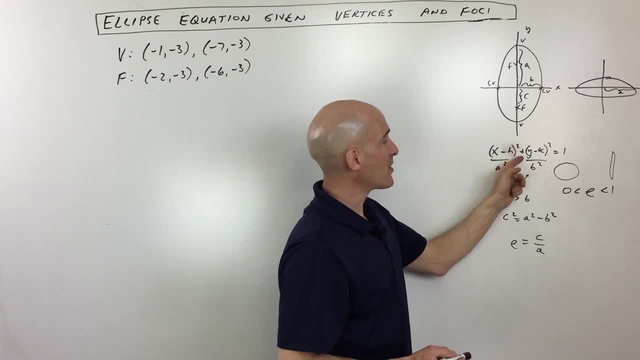 But the general equation you can see is X minus H squared plus Y minus K squared is equal to one And we've got these denominators A squared and B squared. But remember, you know, the A squared and B squared can actually switch. The A is the larger one And that's going to give you the 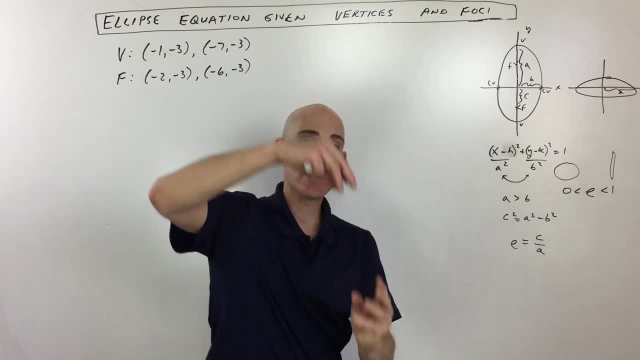 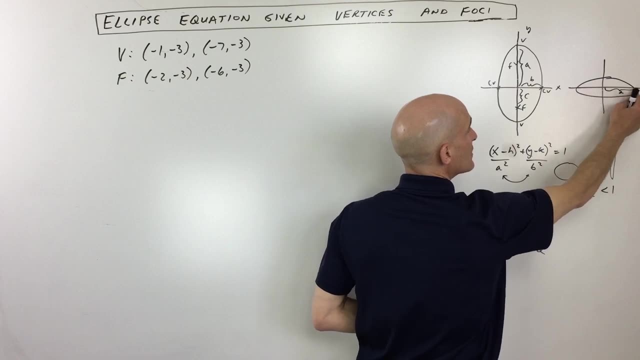 distance from the center to the vertices, And the vertices are going to be on that longer axis, okay, that major axis. So in this ellipse here, A is actually horizontal. It's from the center, left and right. okay, In this case the A would be underneath the. 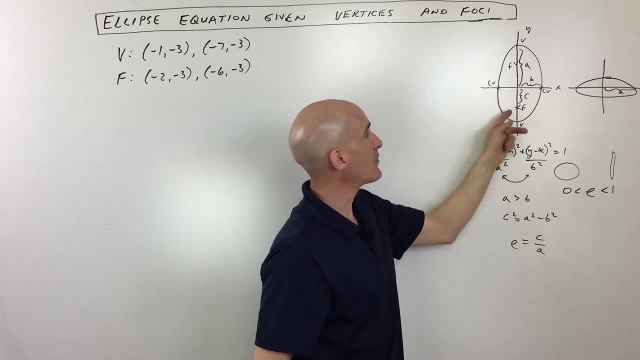 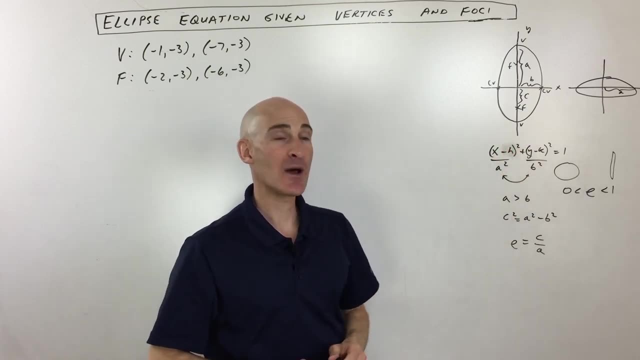 X squared And this problem here, or in this graph, here I should say the A is going to be underneath the Y squared term. okay, And then the H and the K pick up the graph and shift it left and right up and 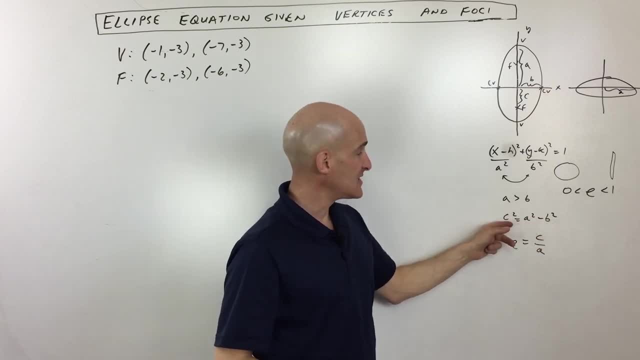 down And then we have an equation that relates A, B and C, That's C squared is equal to A squared minus B squared. okay, Kind of like Pythagorean theorem, but you're subtracting, And then eccentricity is defined as C divided by A. okay, So sometimes you have problems that talk about. 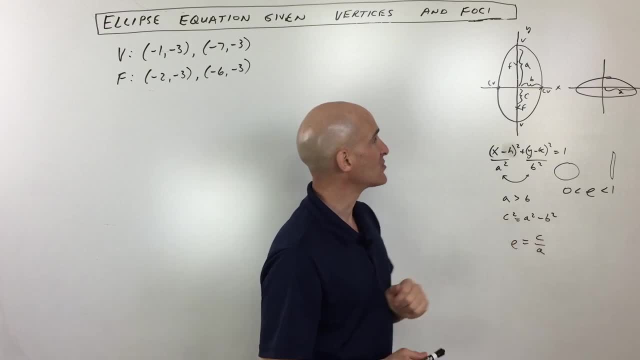 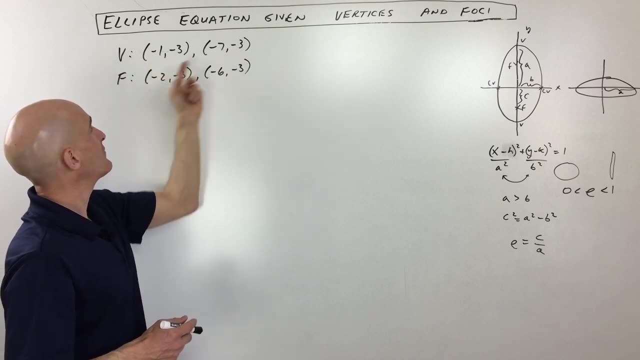 eccentricity In this problem. we're not really going to work with that, So I'll just kind of skip over that for right now. But let's see what they give us here. They give us: the vertices are negative 1, negative 3, negative 7, negative 3, and the 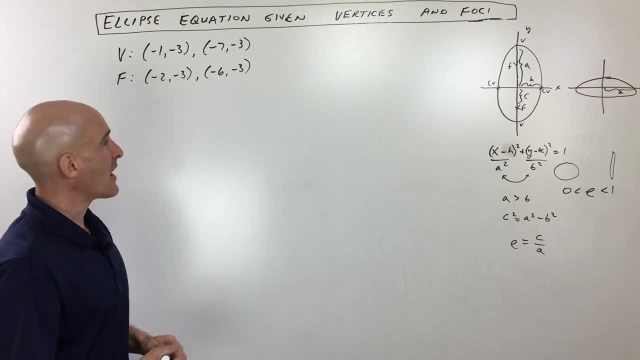 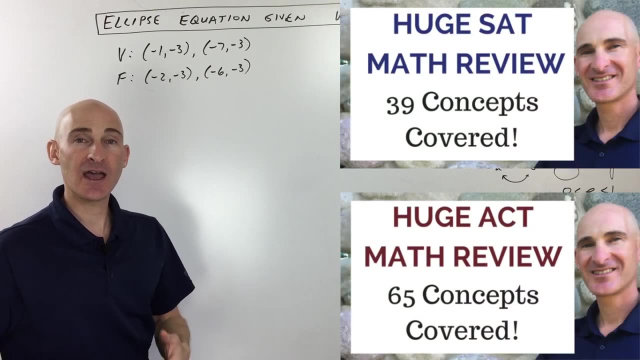 foci are negative 2, negative 3, negative 6, negative 3.. So I'm going to sketch a graph of that. But I wanted to mention, before I get into this problem further: if you're preparing for the ACT or the SAT and you want additional help, check out my two video courses that I put together for 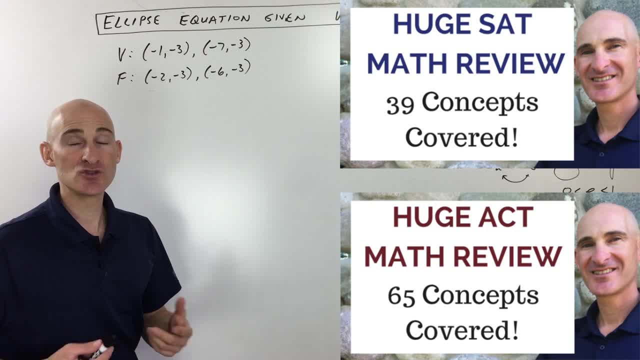 you to help you boost your score. you know and improve your understanding. you know and do better on those tests overall. I go through a teaching section. We have example problems. There's opportunities for you to practice And it goes over some concepts and expected problems that you would likely see on those tests. 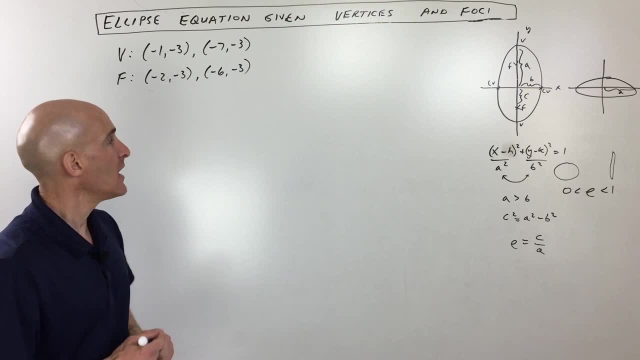 So if you're preparing for those, definitely check out those video courses. But let's continue with this problem. What we want to do is we want to sketch these points here to get an idea of what this graph looks like. So we've got negative 1, negative 3, right there, That's. 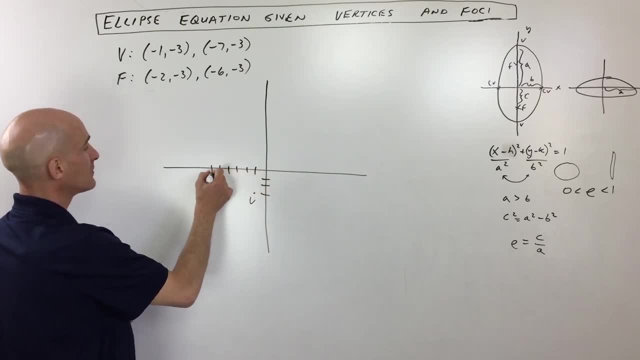 the vertex And we also have a negative 7, negative 3.. That's our other vertex right there, And then halfway in between those vertices is the center point. So one way to do that is to add the axis together and divide by 2.. So that's negative 8 divided by 2. 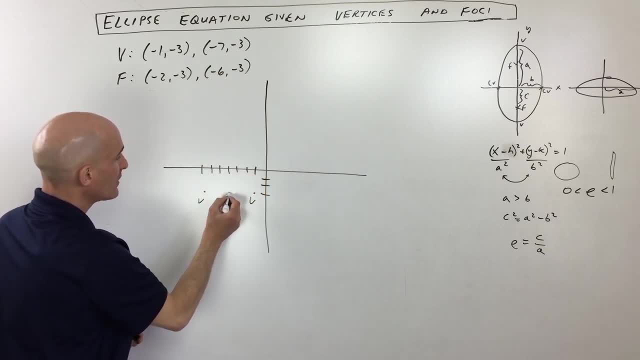 would be negative 4.. So you can see 1,, 2, 3, negative 4, negative 3.. That's our center, So I'll just write that down. so we have that Okay. now the foci are at negative 2, negative 3 and negative 6,. 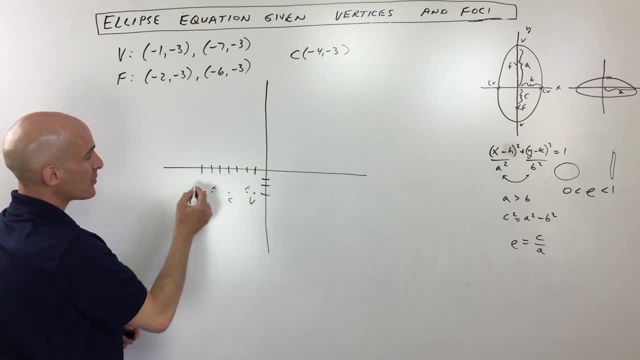 negative 3.. Okay, so there's our foci right there, So you can see our ellipse is going to be longer in the horizontal direction. okay, because the vertices and the foci are on that major axis right. So so far what we have. let's see if we can write down what we have. We've got x minus. 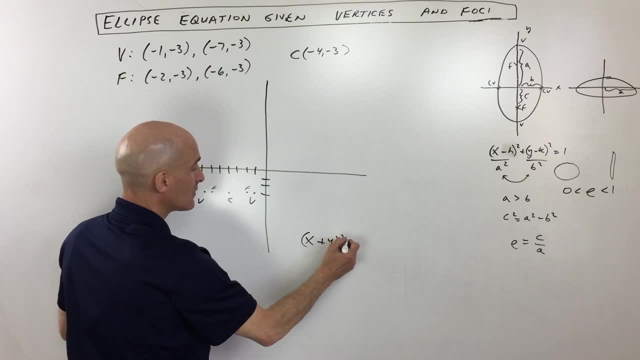 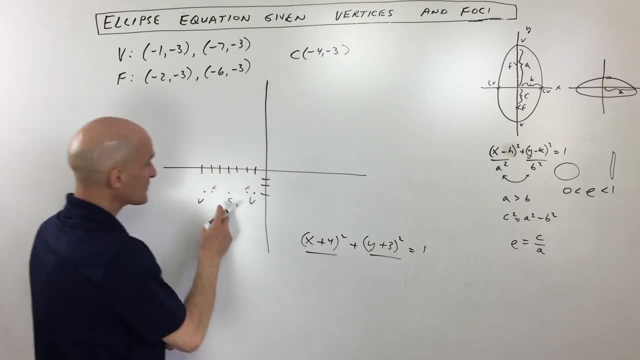 negative 4,, which is x plus 4 squared plus y minus negative 3,, which is y plus 3 squared, is equal to 1.. The distance from the center to the vertex. we call that distance a okay, And so what? 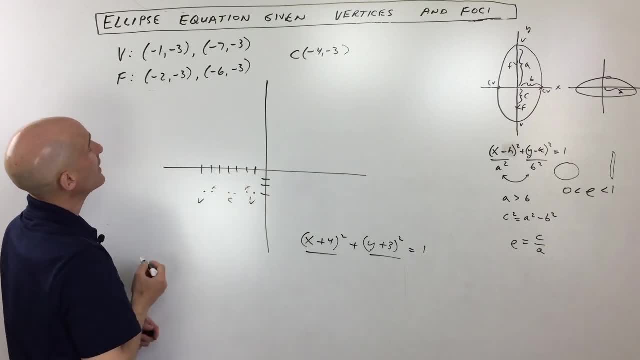 is that distance? Well, you can see it's 1,, 2,, 3,, okay, So that's going to be 3 squared, which is 9.. Now notice, I'm putting that underneath the x because that's going in the. 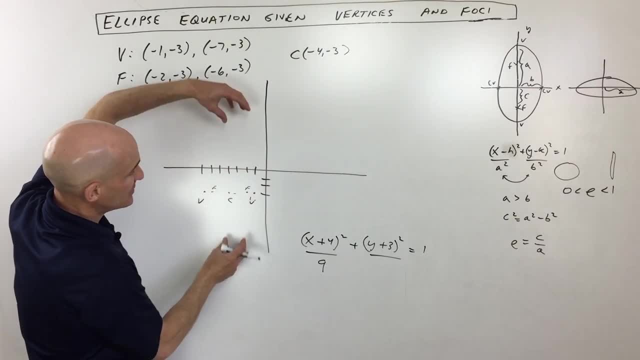 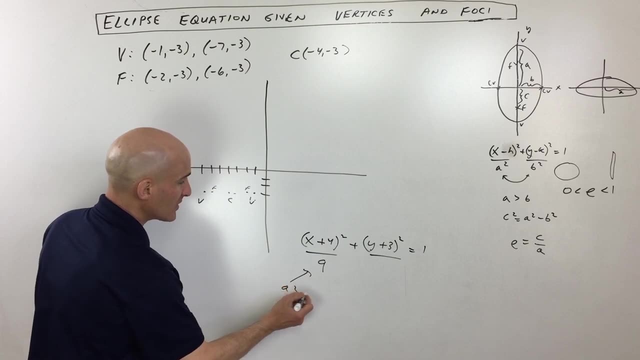 x or horizontal direction. okay, If it was going like this direction, it was longer. in the vertical direction it would go underneath the y, okay, So we've got our a squared Now what we're looking for is our b squared right there. So remember, there's an equation that relates all those. 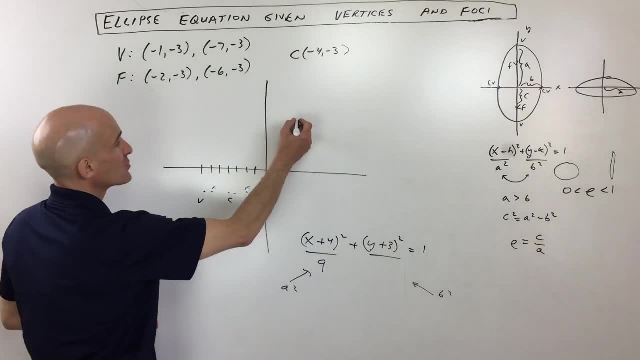 together It's c squared equals a squared minus b squared. So let's go ahead and do that. So c squared is equal to a squared minus b squared. c, remember, is the distance from the center to the focus. In that case, you can see, it's 2.. So 2 squared is 4.. a squared, we figured out was 9,. 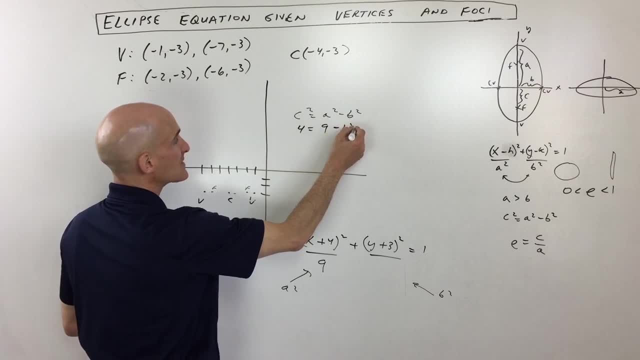 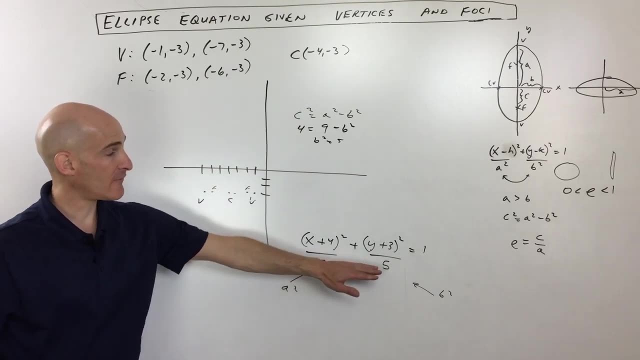 right, Because that's the distance from the center to the vertex, squared minus b squared. So you can see that b squared is equal to 5 if you solve this equation. So this is going to be 5, right there? Now, if you want to take the graph a little bit further, take the square root of 5,. 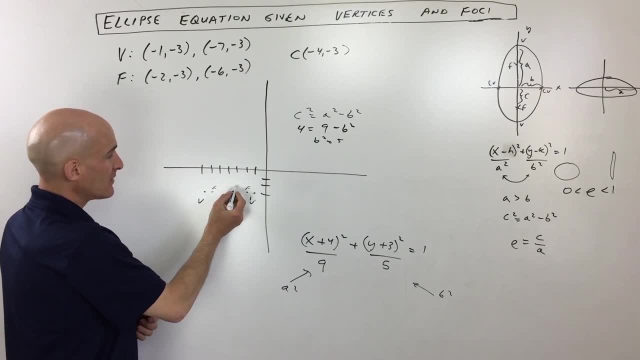 which is about what is that? A little bit over 2, right. So if I go up, let's say a little bit over 2,, right about there down a little bit over 2, that's going to be our graph, right there Pretty. 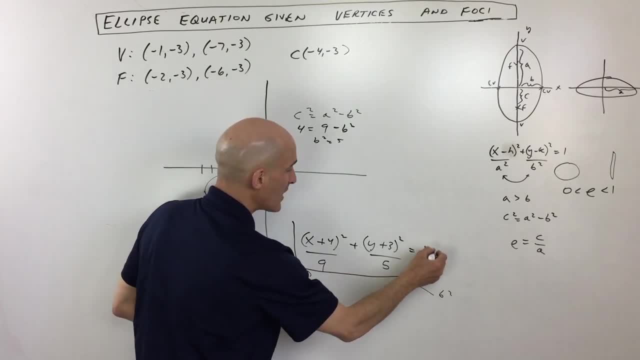 good sketch, okay, But what we were after in this problem was the equation of the ellipse, and that's what we have here. So we're going to go ahead and do that. So we're going to go ahead and do that We have right here. So I hope this helps you understand how to find the equation of an ellipse.